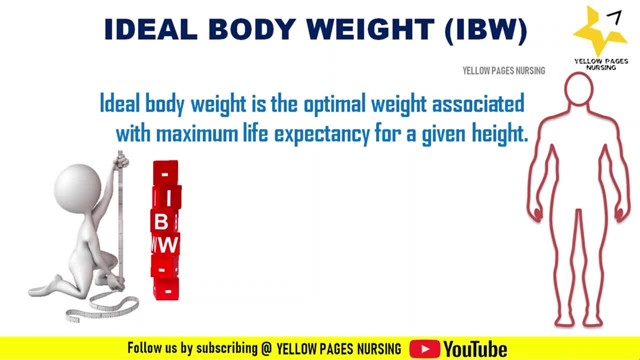 the optimal weight associated with maximum life expectancy for a given height. In short, we say it as IBW or predicted body weight. This measurement is useful for comparing a person's actual weight against a recommended weight based on height. What are the clinical uses of ideal body weight? 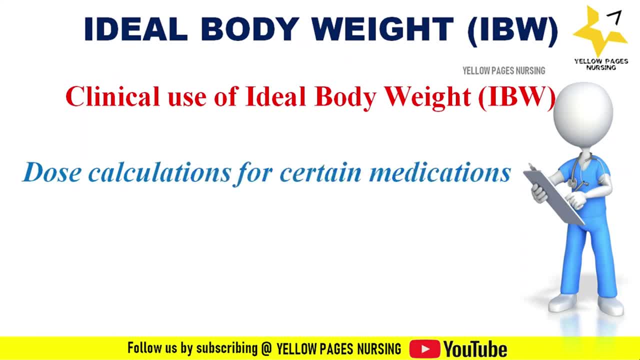 It is used for dosage calculations for certain medications like chemotherapy, anesthetic drugs, etc. In nutrition, protein requirement of a patient is calculated using ideal body weight. Creatinine clearance can also be calculated using ideal body weight. Tidal volume is also calculated using ideal body weight. Now what do we need to calculate ideal body weight of a patient? 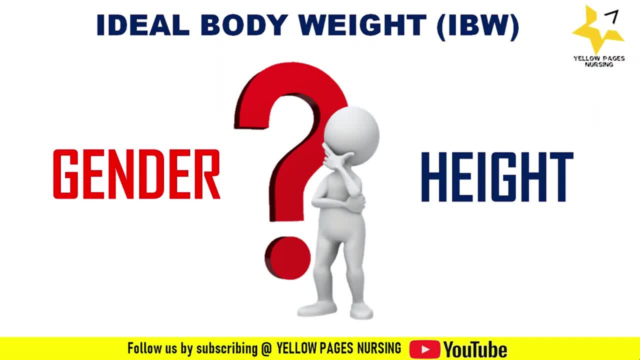 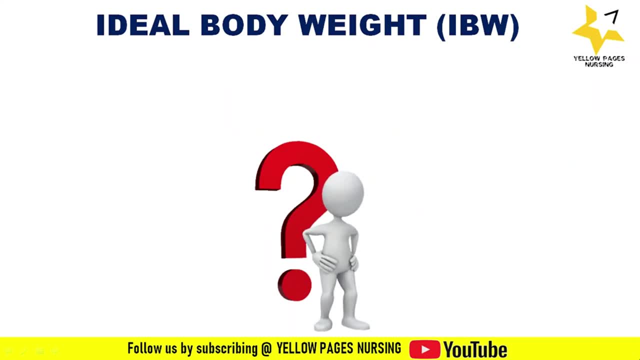 All we need is height and gender of the patient to calculate the ideal body weight. Let's do it with an example: Calculate the ideal body weight of a man who is 160 cm in height. Here, gender is man and height is 160 cm, and these are the information needed. 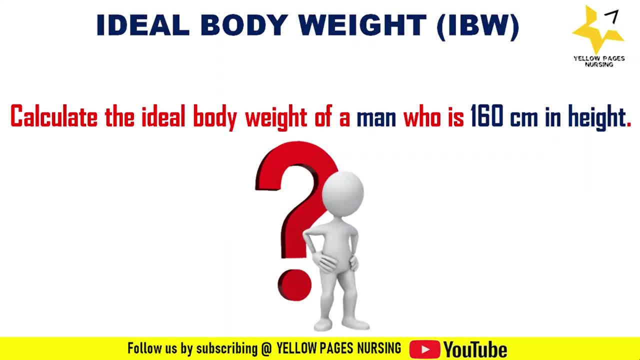 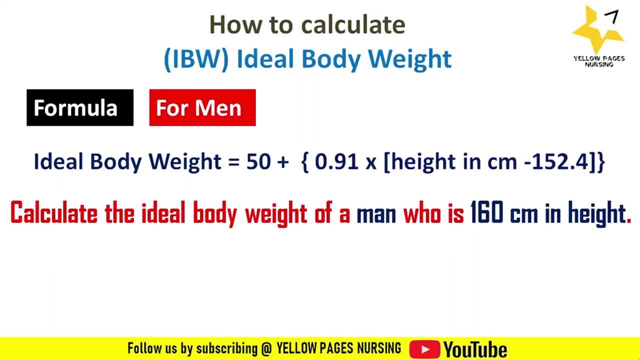 for calculating ideal body weight. Now the formula to calculate ideal body weight for men is: ideal body weight is equal to 50 plus 0.91 into height in centimeter minus 152, point four. Now look into the example: ideal body weight is equal to 50 plus 0.91 multiplied by 160 minus 152.4. 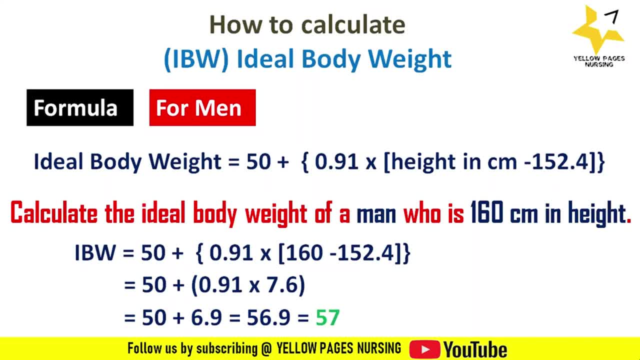 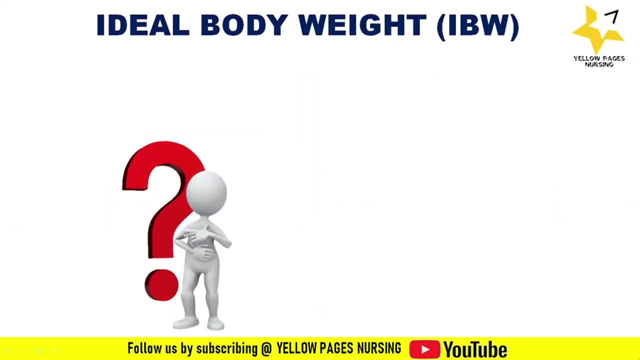 which gives the answer 57. so ideal body weight is equal to 57 kilogramme. Next example is calculate the ideal body weight of a woman who is 160 centimeter in height. Here gender is woman and height is one sixty nine君 seu, and height can be Alzchter ung looks free if 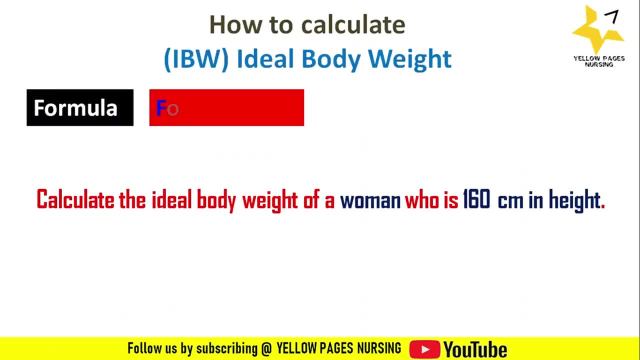 centimeter and the formula to calculate ideal body weight for women is: ideal body weight is equal to 45.5 plus 0.91 multiplied by height in centimeter minus 152.4. and getting into the example, we get: ideal body weight is equal to 45.5 plus 0.91 multiplied by 160 minus 152.4. 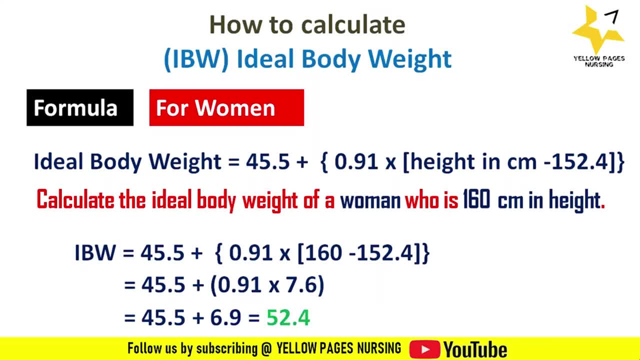 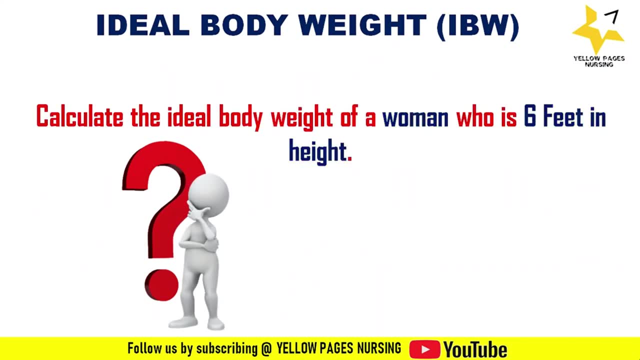 and this gives the answer 52.4. so ideal body weight is equal to 52.4 kilogram. let's look into another example. calculate the ideal body weight of a woman who is six feet in height. when you notice here, the gender is a woman and height is given in feet. what we need to do is we need to. 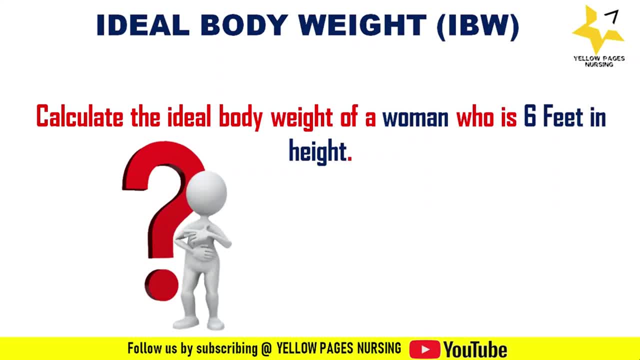 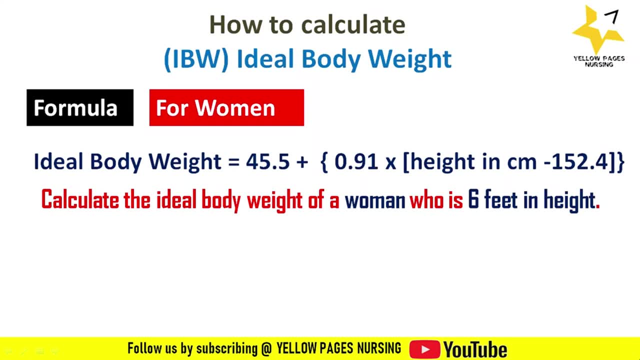 convert feet into centimeter in order to calculate ideal body weight. you now let's do this calculation. the formula for ideal body weight for women is: ideal body weight is equal to 45.5 plus 0.91, multiplied by height in centimeter minus 152.4. so first we need to do is: 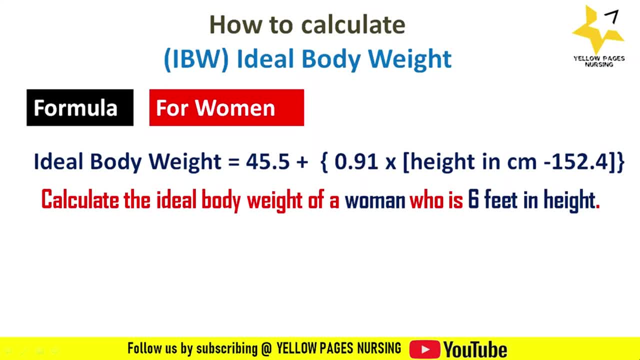 convert feet into centimeter. here the height is six feet, so one feet is equal to 30.48 centimeter. so six feet will be six multiplied by thirty point forty eight, which gives 182.. eight centimeter. so applying this into the formula, ideal body weight is equal to 45.5 plus 0.91 multiplied by. 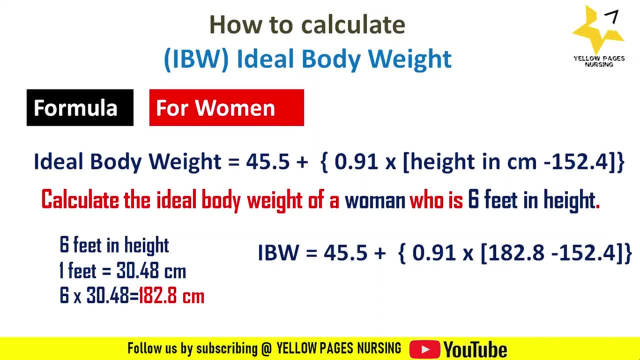 182.8 minus one fifty two point four, which gives the answer seventy three. so the ideal body weight will be 73 kilogram. so the formula we need to remember for calculating ideal body weight is: ideal body weight will be 73 kilograms. so the formula we need to remember for calculating ideal body weight is: ideal body weight is: 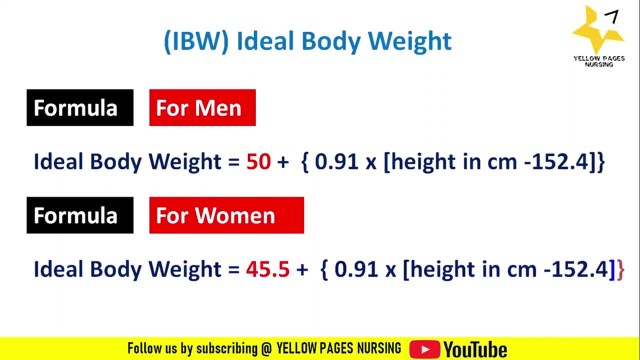 body weight for men is equal to 50 plus 0.91, multiplied by height in centimeter minus 152.4, and ideal body weight for women is 45.5 plus 0.91 multiplied by height in centimeter minus 152.4. 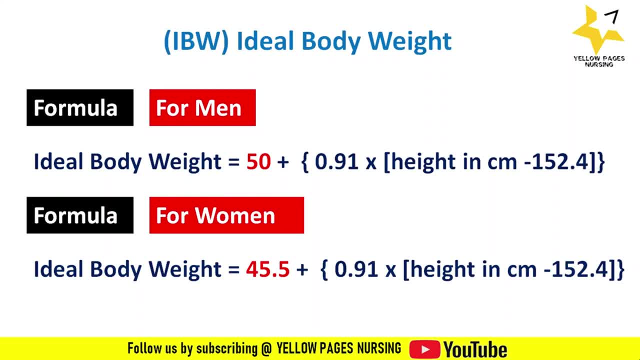 the only difference is we add 50 in case of men and 45.5 in case of women. and one more thing we need to remember is if the height is given in feet or inches, we need to convert this into centimeter in order to be applied in this formula. now few examples for your practice. calculate the ideal.